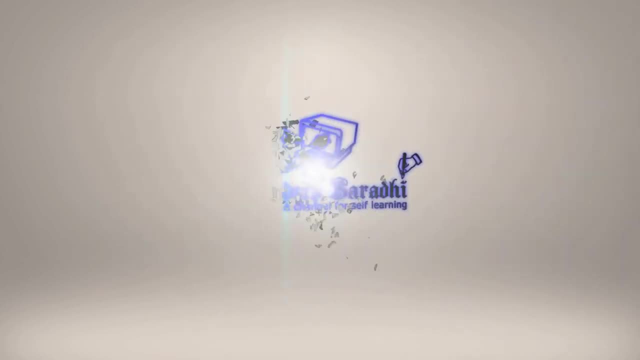 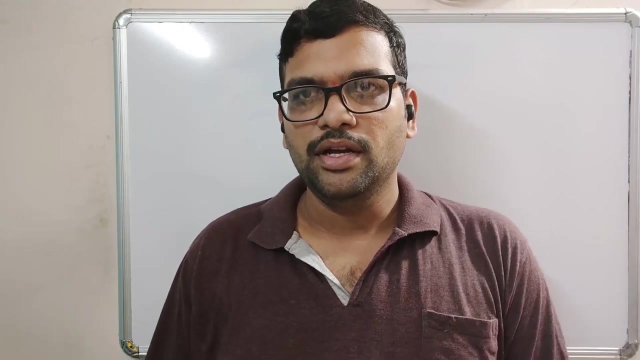 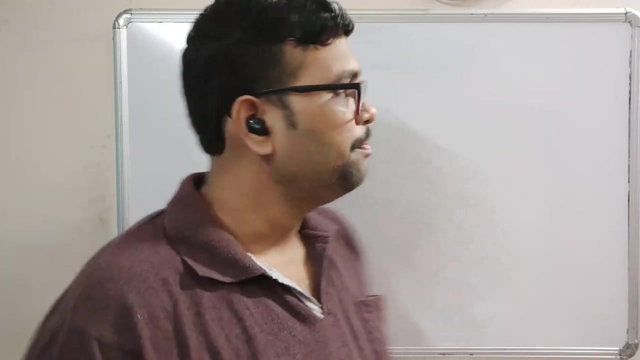 Hello friends, welcome back to our channel. So in the previous session we have discussed about how to install the matplotlib, So in IDLE, as well as the Jupyter, And in today's session we'll see some introduction on this matplotlib. So introduction to matplotlib. 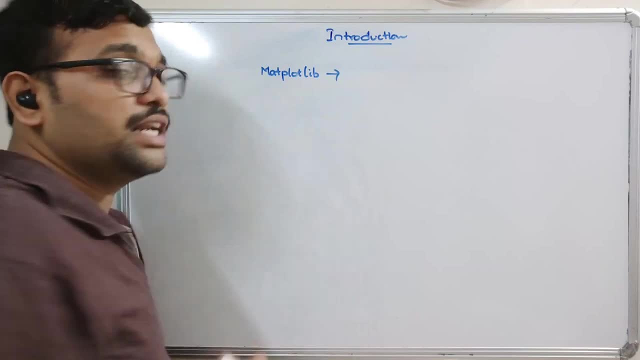 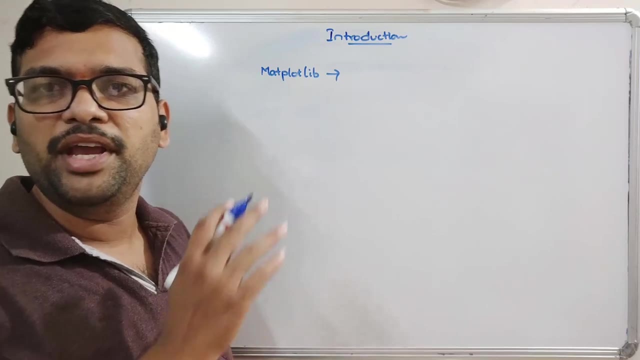 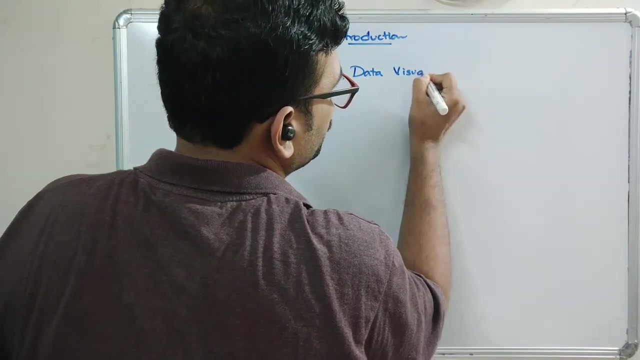 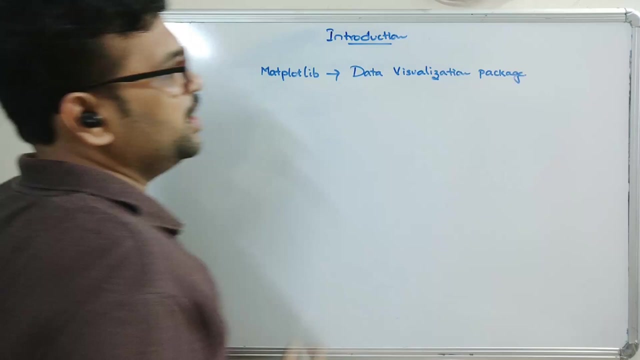 So matplotlib is a data visualization package in Python. So if you want to visualize the data in terms of graphs or charts, we can make use of this matplotlib. So this is a data visualization package, The package or a library, right? So here we'll be having two modules. One is a mat, sorry, 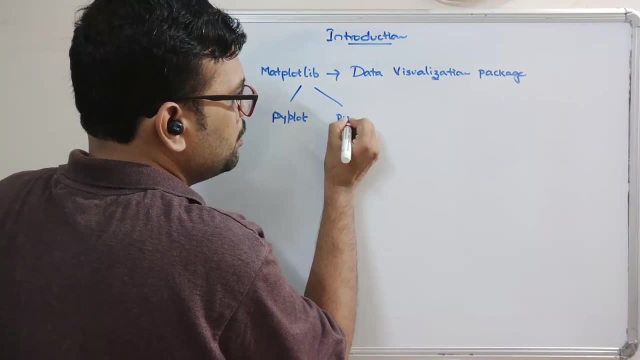 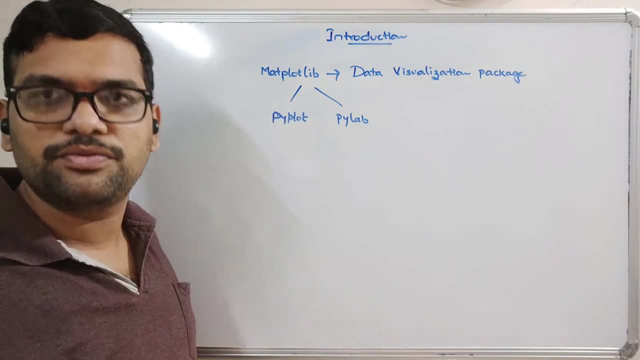 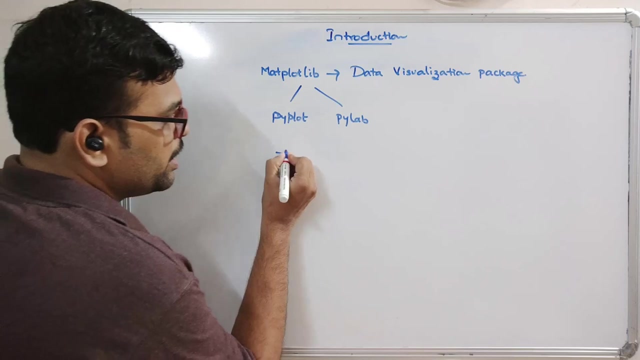 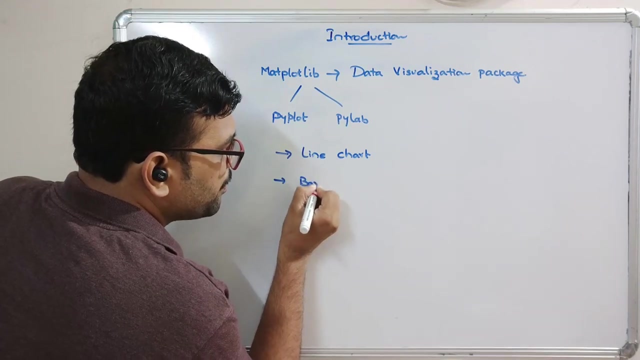 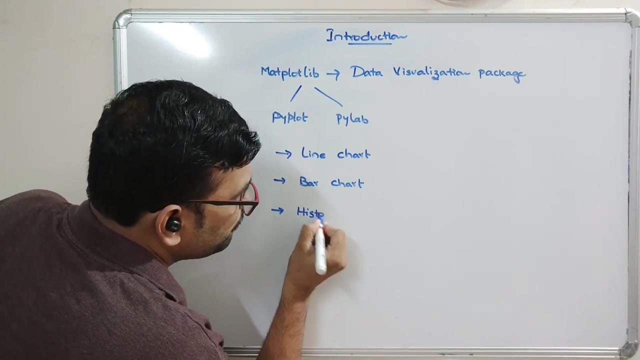 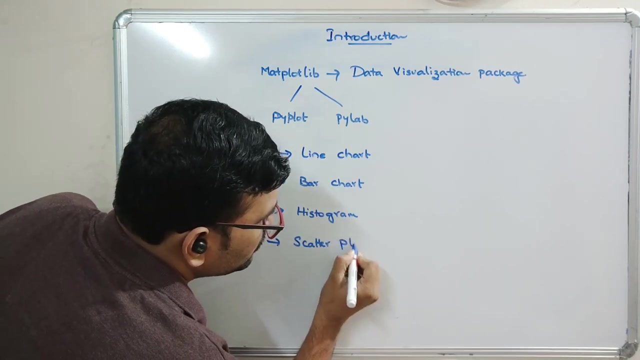 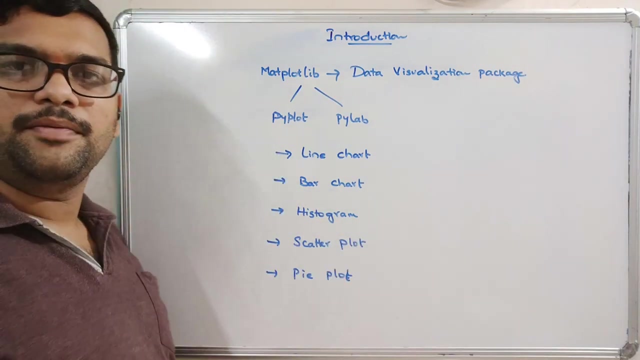 pyplot, Another one is a pylab. So by make use of this pyplot and pylab, we are going to create the different types of charts. Now the question is what type of charts we can represent by using this matplotlib And line chart. Similarly, bar chart, Histogram, Scatterplot, Pyplot, Pyplot or chart. Okay, 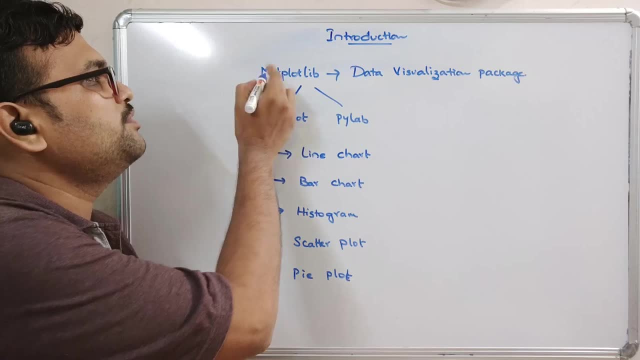 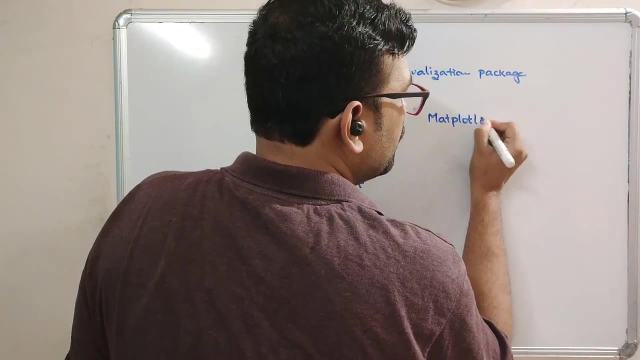 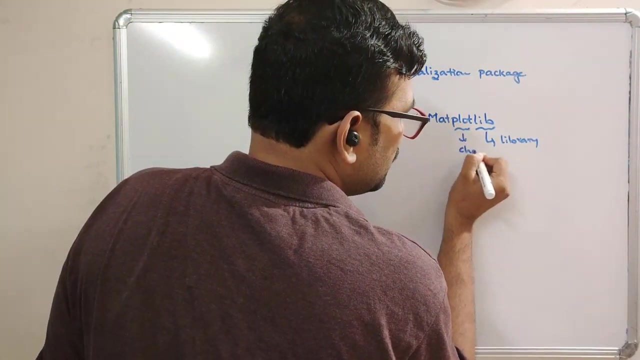 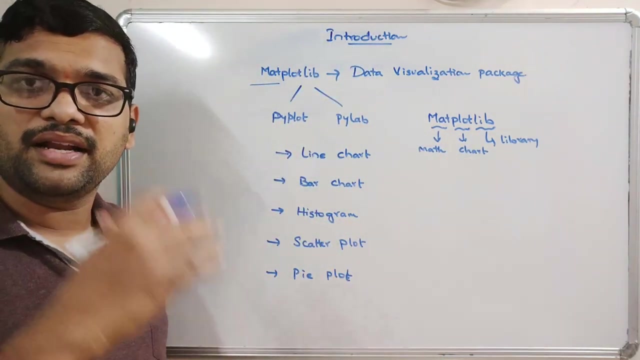 So these many graphs we can, We can represent with the help of this matplotlib. So you can observe here Mat Plot Lib. So here this lib stands for the library, Plot stands for a chart And mat stands for some mathematics. Okay, So whatever the result we are getting from some mathematical expressions, 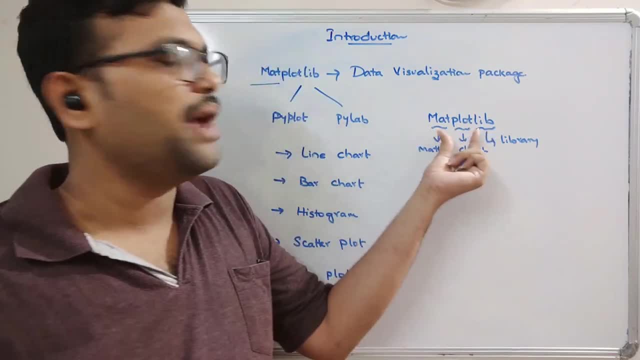 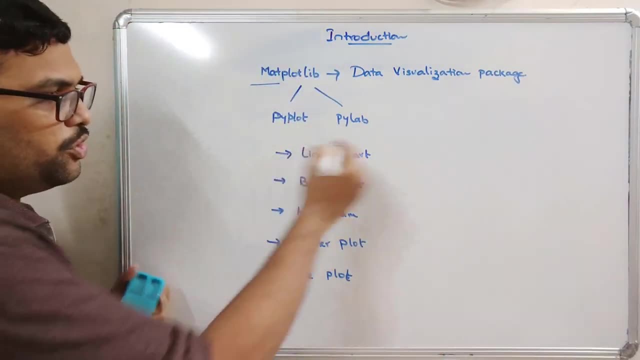 that can be plotted with by using this library called matplotlib. Okay, So what we are getting from some mathematical expressions that can be plotted by using this library called matplotlib. Okay, And just, I will show you all these charts, how this line chart will be represented, how. 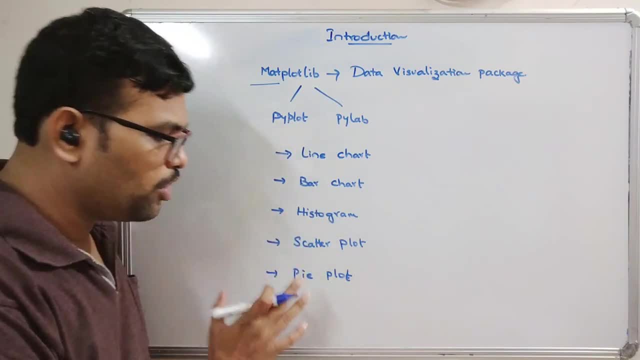 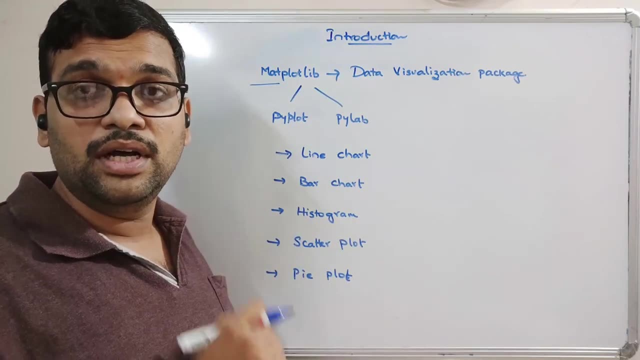 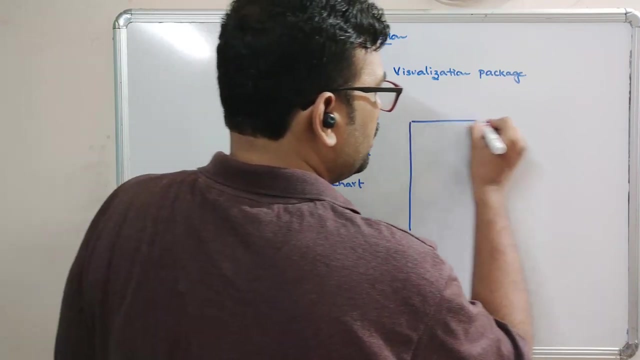 this bar chart will be represented how the histogram, how the scatterplot and how the pyplot in the system. So meanwhile I will give you a few basic introduction about the chart. So basic requirements we can create on the chart. So we know that it's a chart or a graph, Right Chart or a 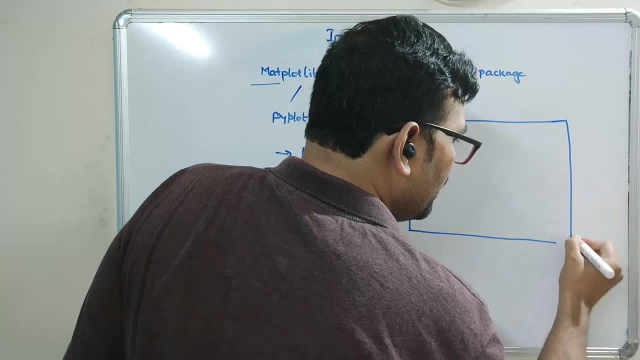 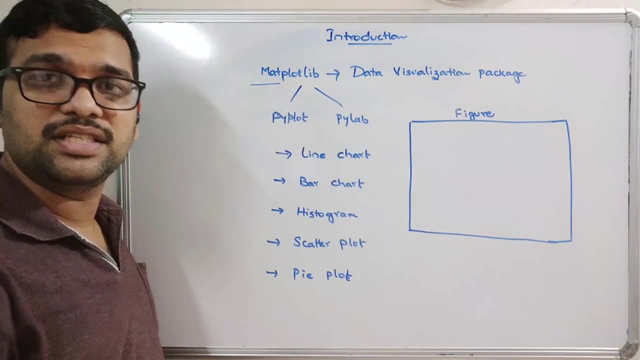 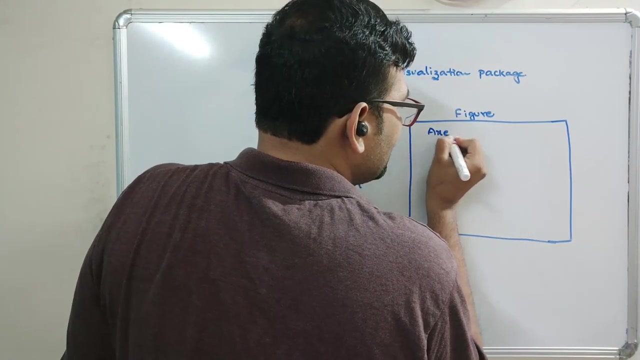 graph. So the place, Okay, So where we are creating these charts is called figure. Figure. Figure is a place where we are giving the charts, Where we have to create the props. Right And inside the figure we will be having the axis. Axis means the place where we are drawing the chart. Okay, 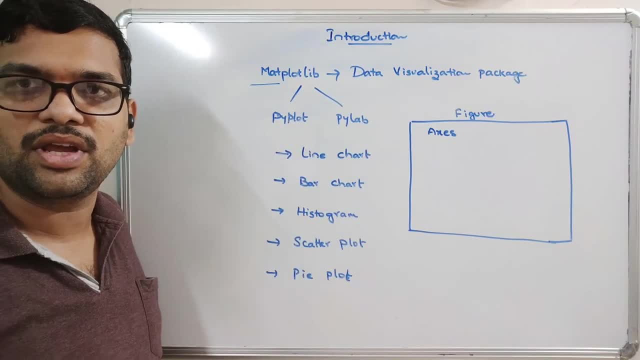 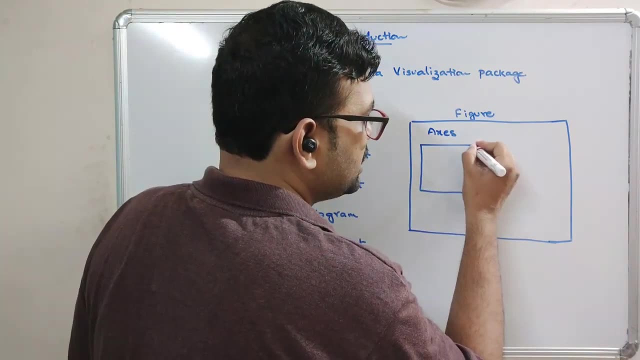 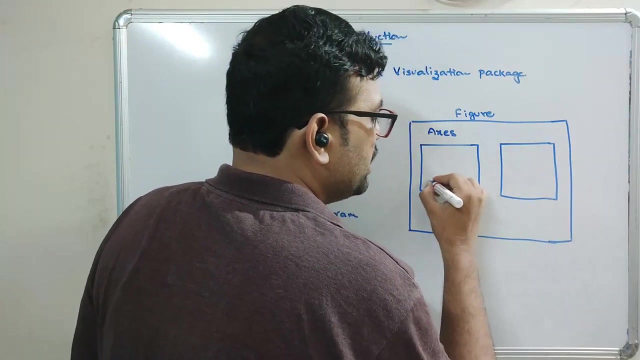 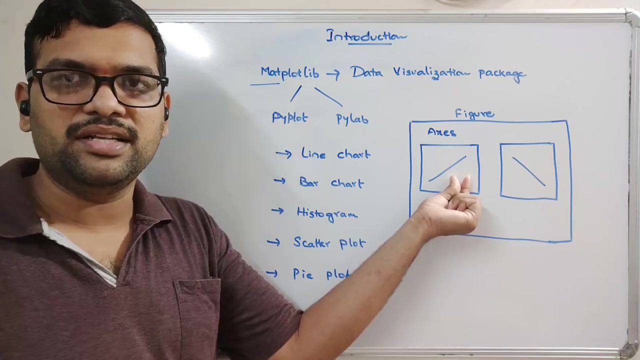 So one figure may have a different axis. Okay, One figure may have different axis. So that means: See one axis and this is another axis, so a figure can have a multiple axis. right, so this is one graph and this is one graph. for example, it's a line graph. okay, it's a line graph, this is one line. 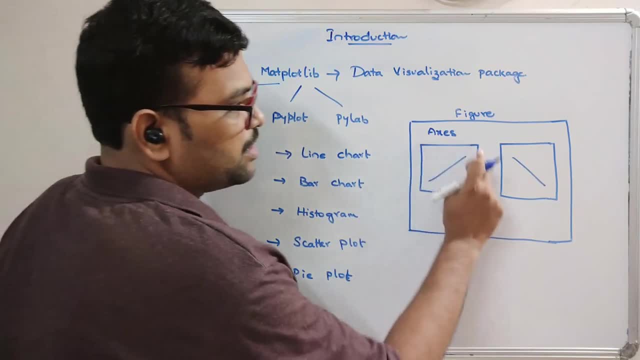 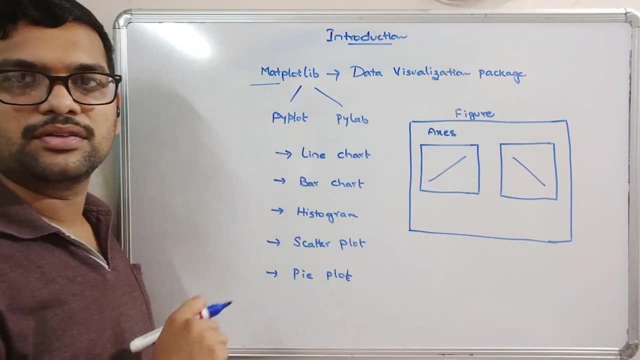 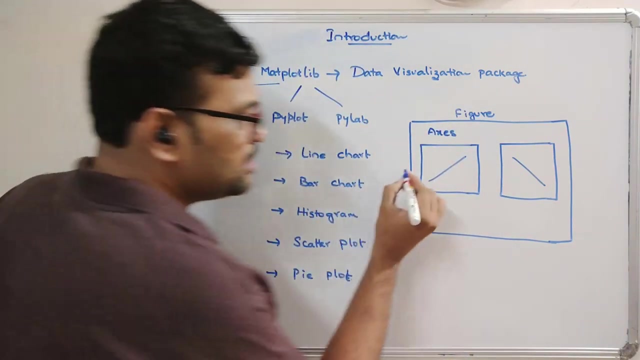 graph and this is another line graph. so this part, this portion, is called axis, so different axis can be written on one figure. so figure is a place outline, okay, outline of the window. and in each axis, in each axis, there will be x axis and y axis. so this is called axis: a, x, i s. 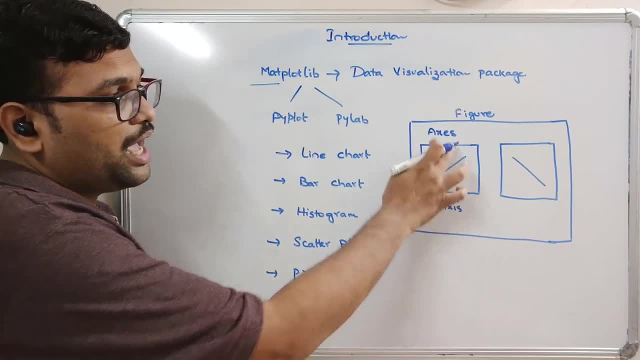 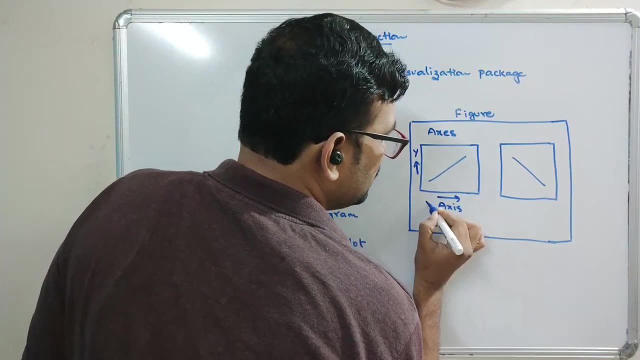 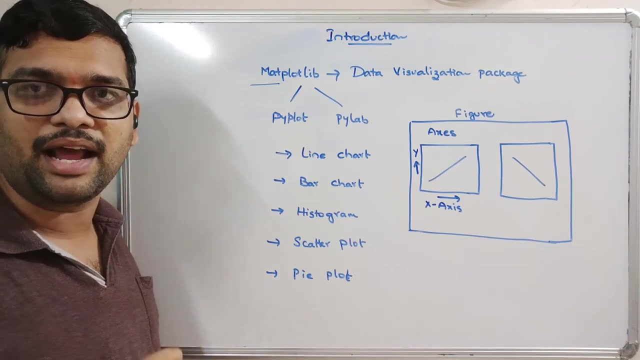 so slight difference. a x i s dimension right. a x e s is nothing but a place where we are drawing the chart. and this is axis, this is y axis and this is x axis right. so each and every axis will be having x and y if it is a two dimensional graph, if it is a three dimensional. 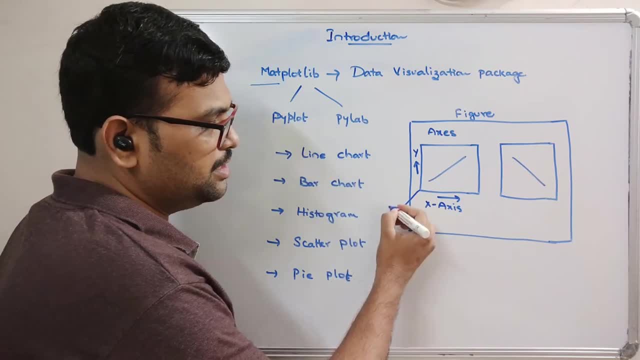 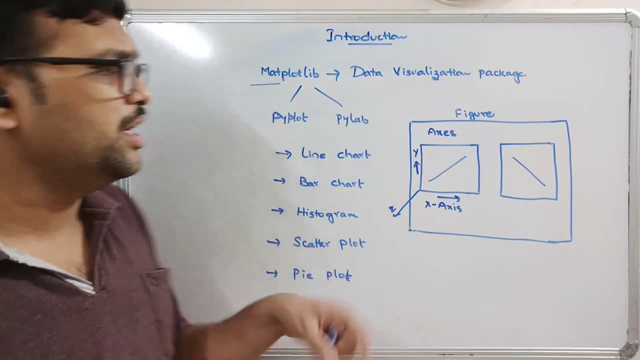 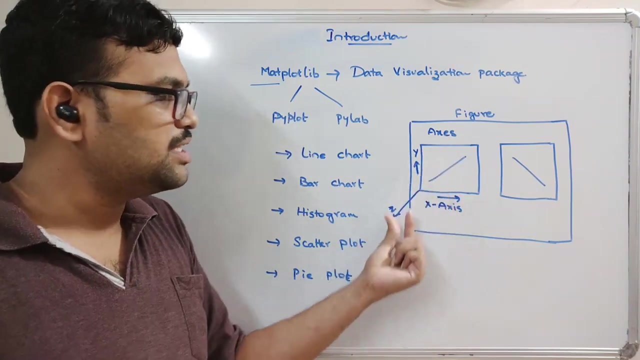 graph we can also represent the third axis, that is, z axis. that is a z axis, so depends upon the graph dimensions of a graph. we need to represent the axis for each axis we have will be having some axis, so x axis, y axis and z axis, and to represent this line 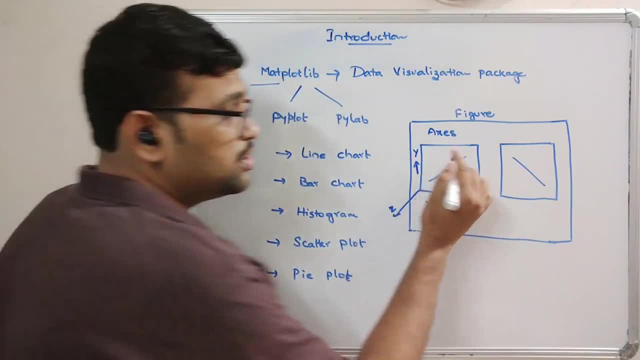 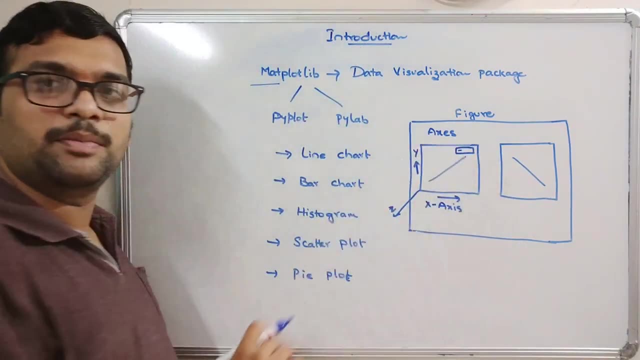 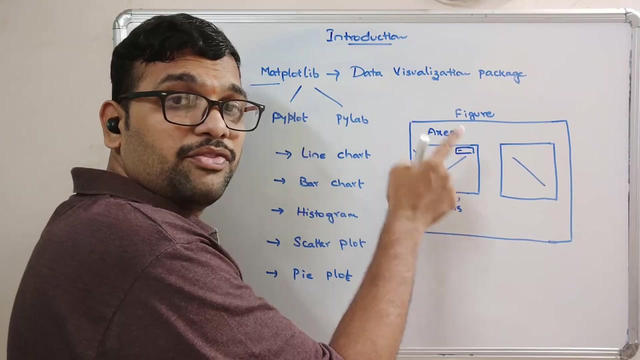 so what? what this line shows that will be called as a legend. so here you can get the square box and here you can represent the line. that is the formula of this line or the functionality of this line, right? so if your diagram, if your chart is having some two lines, you can represent each line with a different. 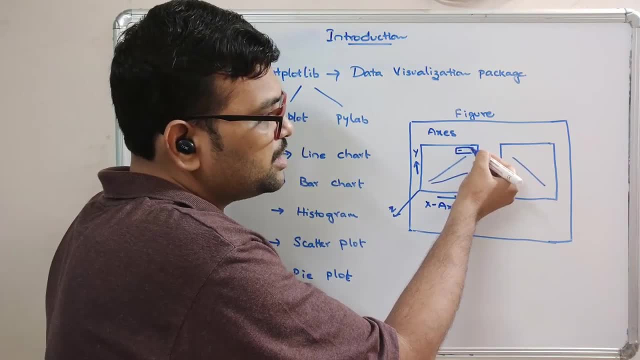 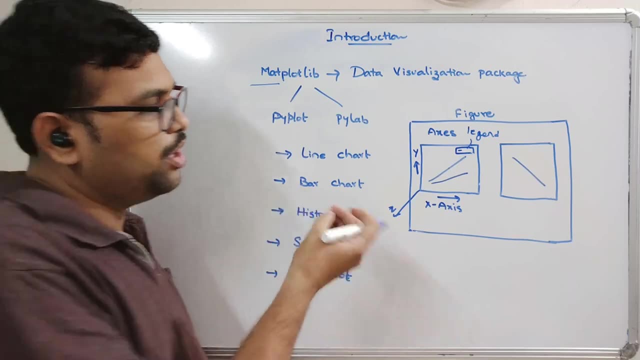 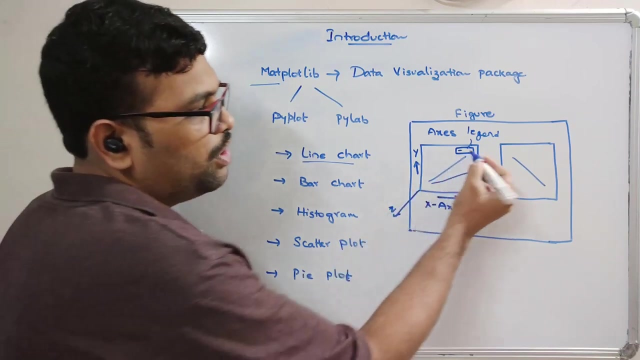 color and you can represent that colors in this square box. this is called legend legend. so I will show you by executing a small line chart in the next session. so meanwhile I am telling about the basic, basic things on the chart. so this is called a legend, which represent the functionality of the line chart or a. 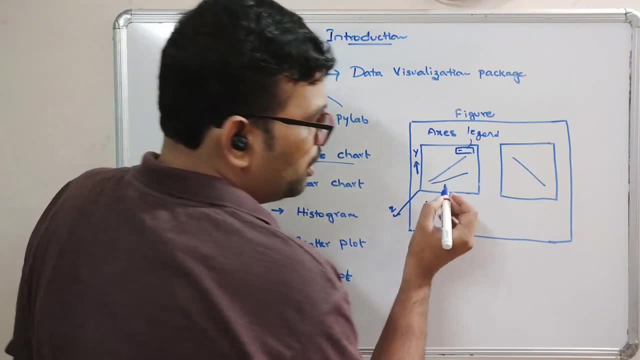 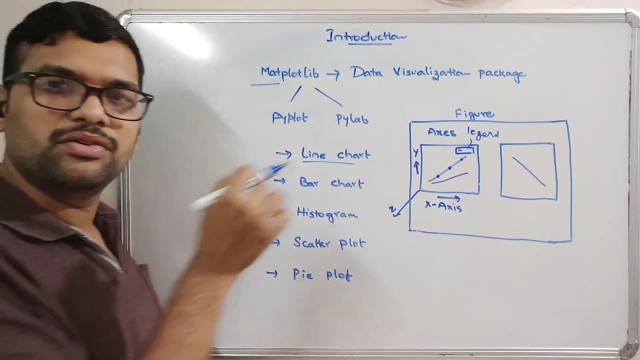 bar chart or a histogram, whatever it may be, and in order to mark the points here, if you want to draw the line or a pie chart, whatever it may be, you need to give some marks right, so these are called as a line chart or a pie chart or whatever it may be. you need to give some marks right, so these are called as. 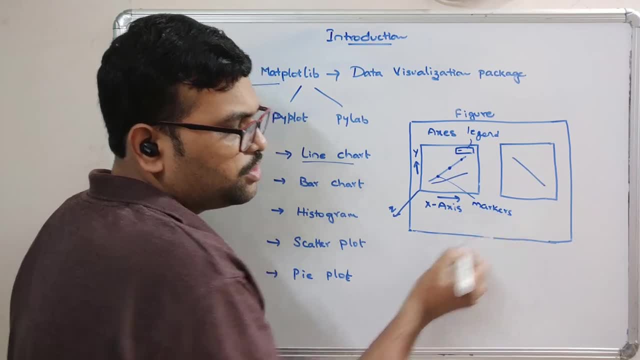 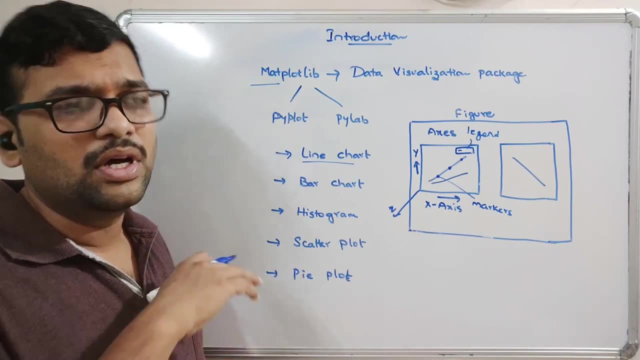 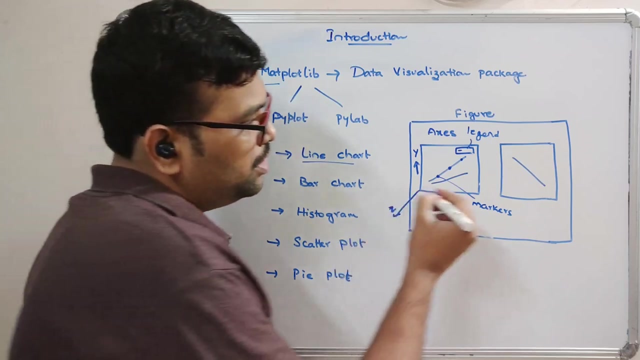 markers. these are called as markers, so we can have a different types of markers. we can represent in the circle, we can represent in a star, we can represent in a pentagon, so different ways we can represent these markers. and also we can change the sizes, we can change the colors, right. so this, this is the markers. 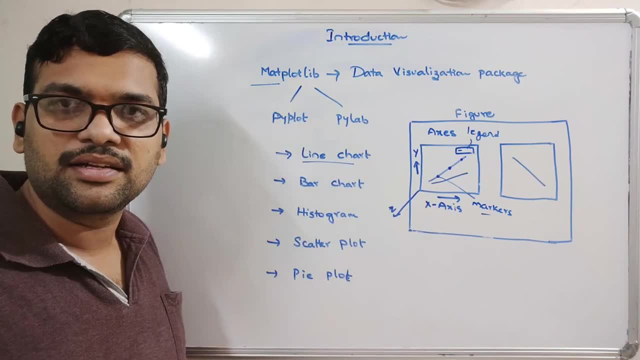 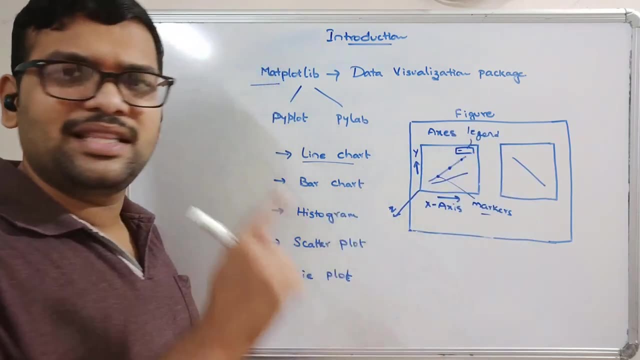 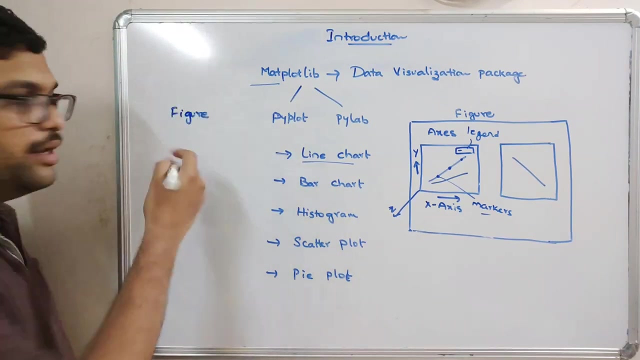 which points the x-axis and y-axis right. so based upon these points only we are plotting the graph. so these are the basic things that we need to know about basic things we need to know before starting the graph. so that is figure, the outline axis, the place we are drawing the chart. so in that we are going with. 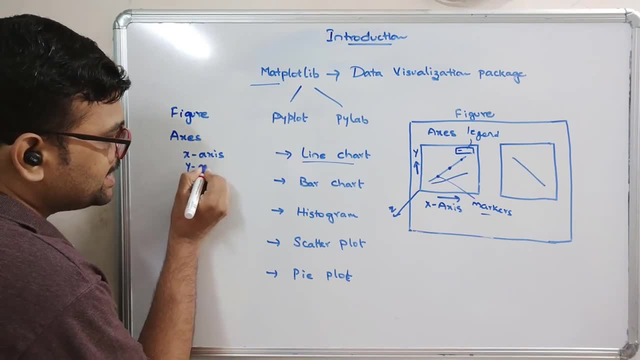 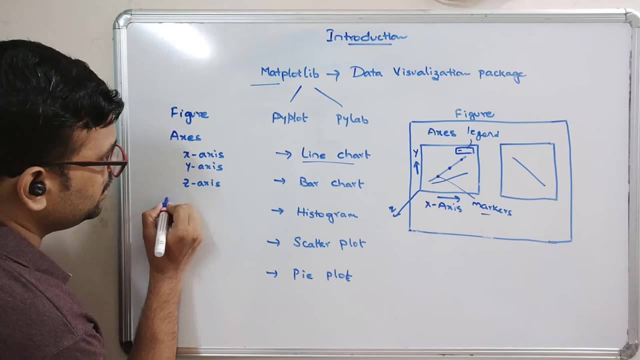 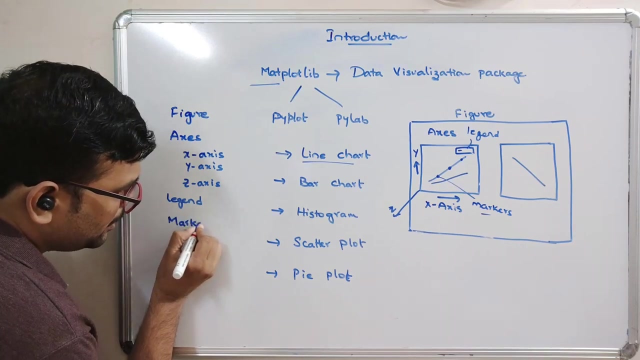 the x-axis and y-axis, and if it is a three-dimensional, it will be a z-axis, and the next we'll see about the legend, so which gives the functionality of that particular line, and then the markers, and then we are going to see about the 2021. we are going to see about the 2021. 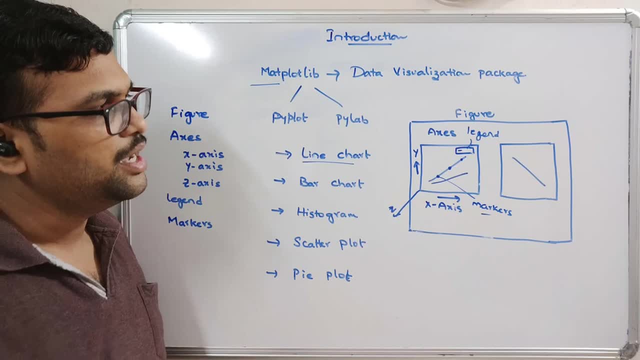 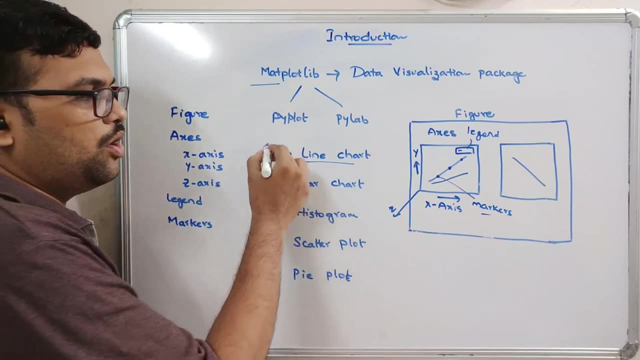 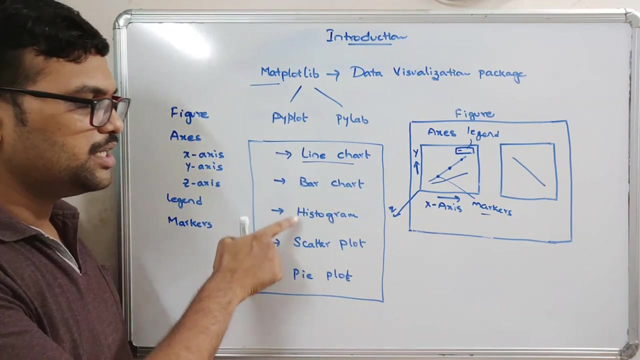 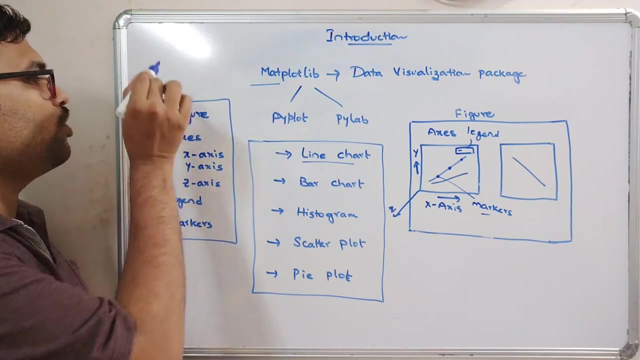 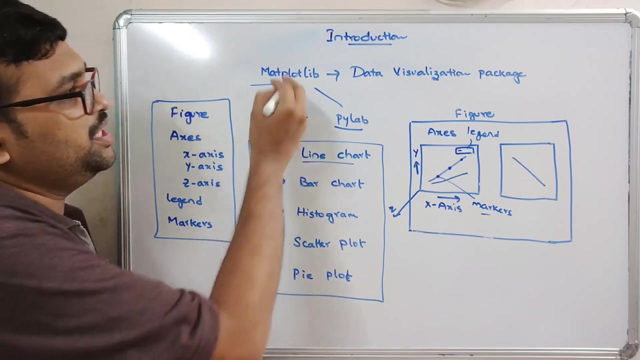 that Senior. we can draw all these charts. these different charts can be drawn by using the map 담당 낮아 이번, number two, to dry this drawing a chart right. and these are the two different modules, two different modules available in this matplot. so now I will show you how the line chart. 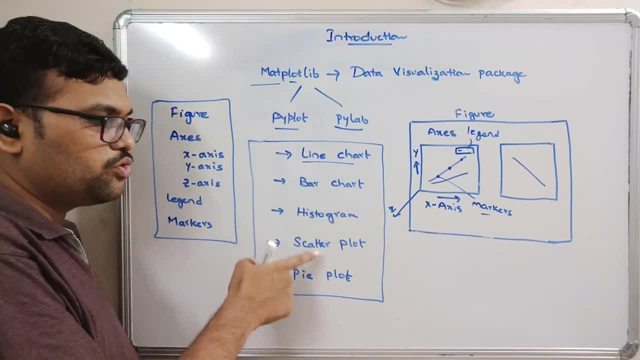 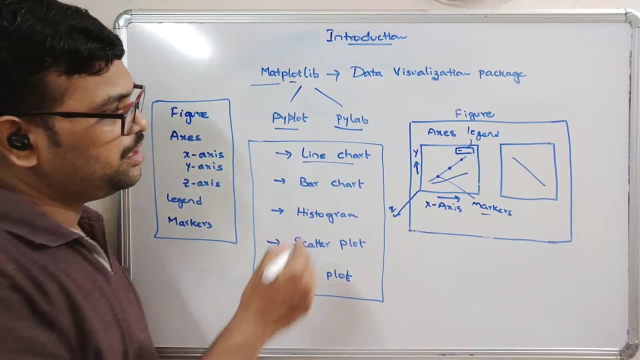 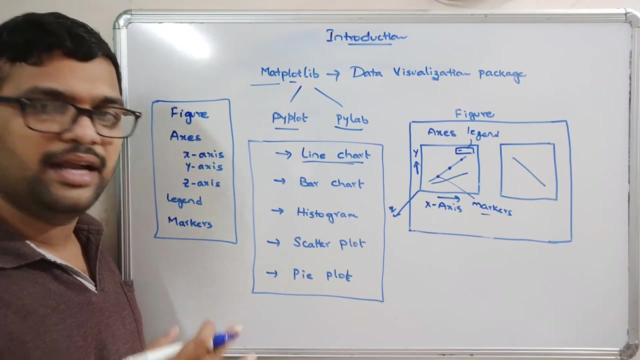 will be represented, how the bar chart will be represented and how the histogram scatter plot and pi plot. okay, so in the next session, from the next session, I am going to show how to draw the line chart. okay, how to plot the line chart and then the bar chart and so on. right now I will show you the. 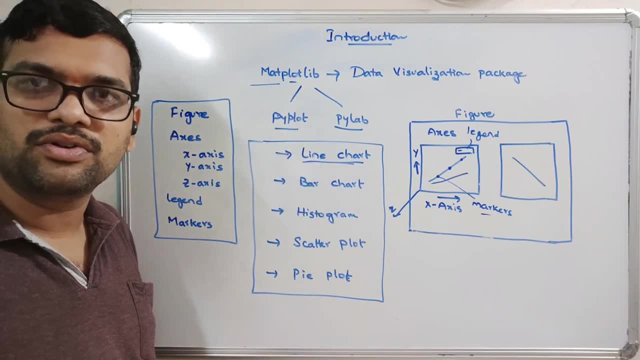 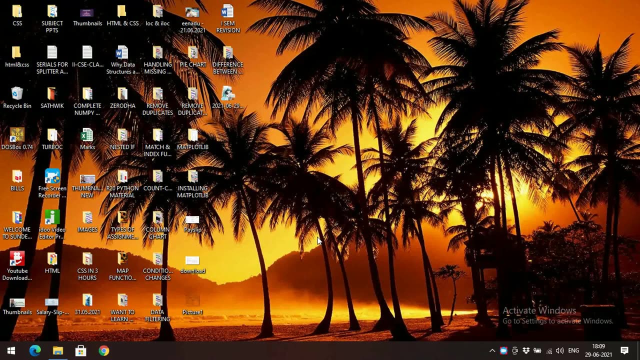 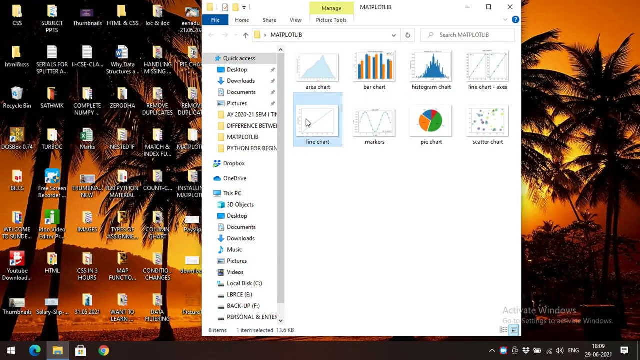 representation of all these charts in the system. so let's move on to the system. hello friends. so just now we have seen the basic terminologies of a graph and what are the graphs- types of graphs that can be drawn with the help of matplotlib. I will show you the thing. so this is an example for the line chart, so the 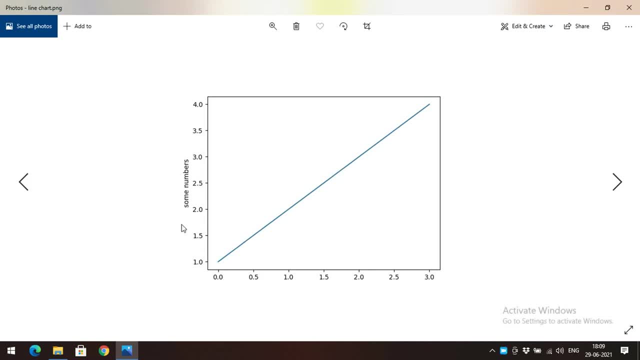 line chart will be like this: okay, in terms of line. so I checked this and the economy ofIE buy 같. and if it isn't three-dimensional, we get a that axis also, and coming to this one is a pile chart. okay, this is a circular representation and there's a scatter plot: the bubbles representation scatter. 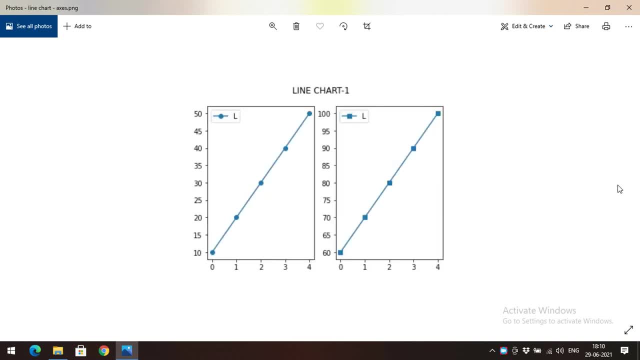 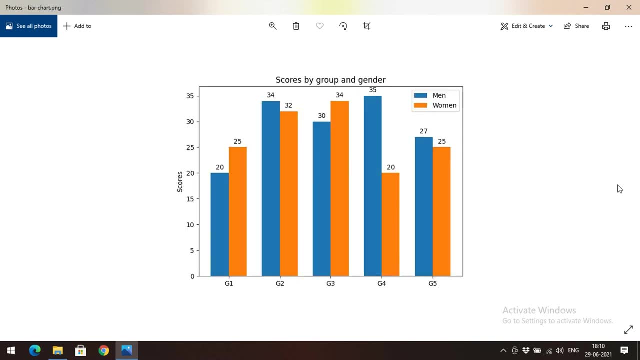 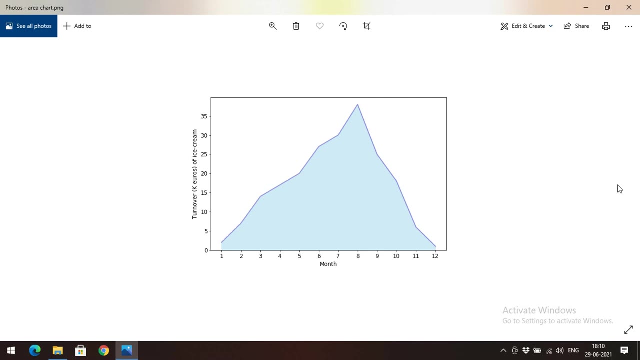 plot, and so this is a histogram representation. so in this way we can represent the data. and this is the bar chart, bar chart, this is the area chart, area chart. so these are the different ways we can represent the graphs. and coming to the basic terminologies, as i have said that, so you can observe here, so this: 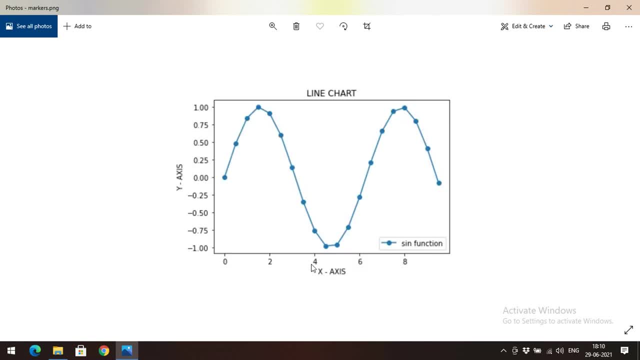 completely known as a figure. okay, the, where we can place, and this is the axis you can observe here. this is one axis, this is one axis. okay, so in the same figure, we are representing two different axes, right, and coming to this one you can observe. so these are the markers. okay, the point in zero. 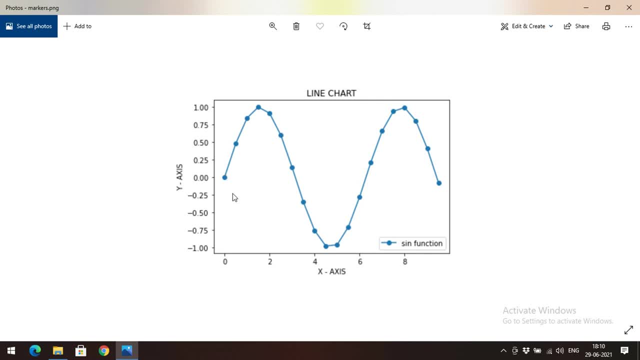 with a zero, it's a marker, one marker, that is a circular representation, and 0.1 it is represented with a 0.5. so that's one type of marker, okay. and again, this is the title line, chart is a title, okay. and these are the axis, x axis and y axis, and this is the legend, so legend. 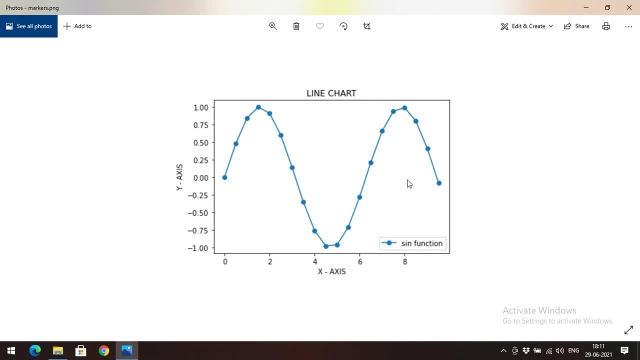 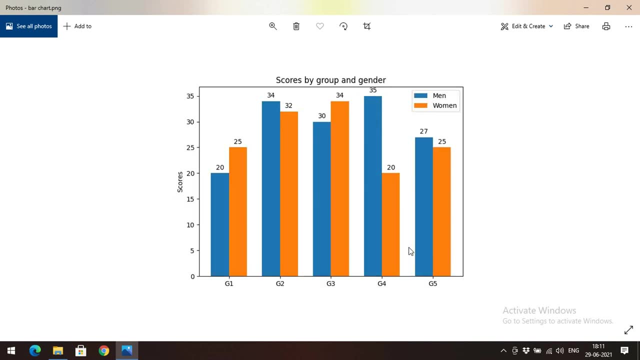 means it shows the functionality of this particular graph. so this is a sine wave. right, this is a sine wave. so if this is a sine wave, so here we are representing it as a sine function. if you observe here, so you can observe: here this is a bar graph and here we are having two different. 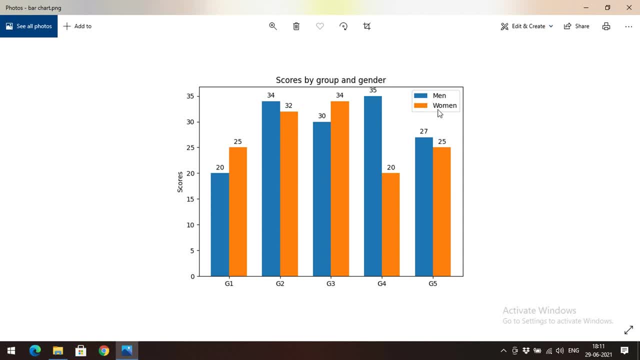 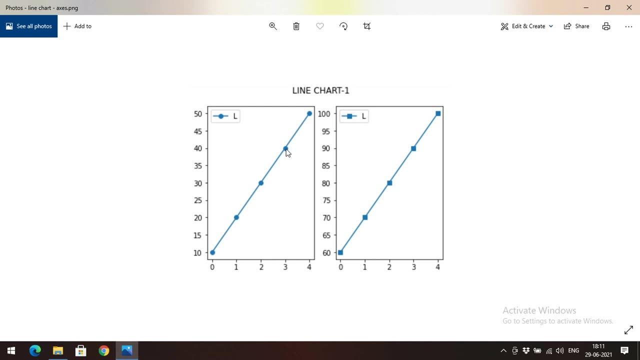 colors: blue represents the men and some orange represents the women. so that is called a legend. okay, gives the functionality of the graph right. so these are the different ways we can represent, and here the representation of the graph is represented by the markers, so these markers can be represented in different. 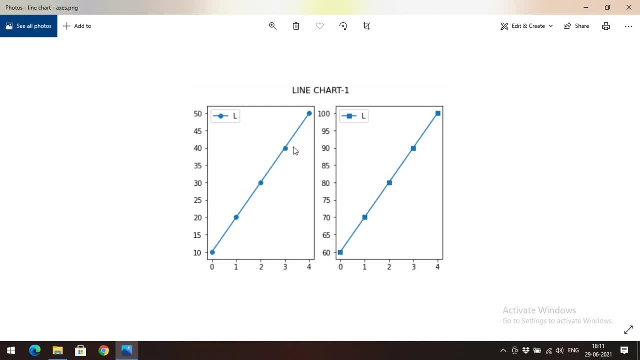 ways, by using circular, circular triangle, square, pentagon, so whatever it may be, and also the lines. the lines can also be represented in different ways: a dotted line, dashed line- okay, like this. we can represent the data in terms of charts, okay, or graphs. so main use of this. 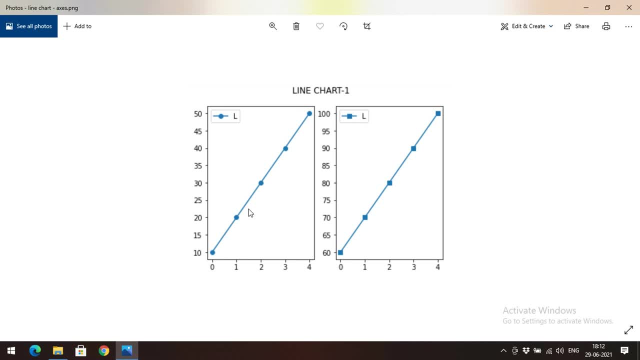 matplotlib is data visualization in order to represent the data in terms of graphs. we are moving with the matplotlib. okay, that's a data visualization library in python. so in this we are going to use the two modules, that is, a pipelot and phylab. so, with the help of 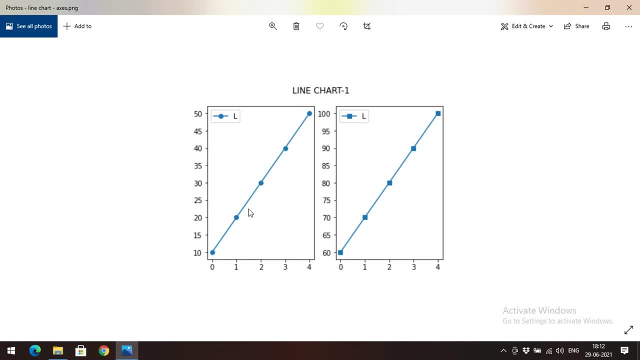 the pipelot and phylab, we are going to draw the graph. so this is all about the introduction. so hope you understood this introduction. if you are having any doubts regarding this session, so feel free to post your doubts in the comment section. definitely will try to clarify all your. 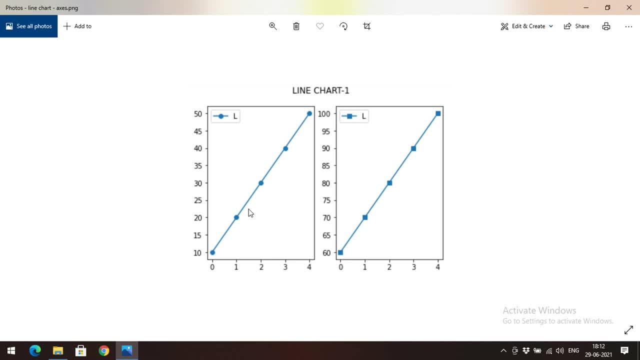 doubts, and in the next session we will start one by one. So first we will see the line chart, then bar chart, then pie chart. So like this, in each and every session we are going to discuss about these charts. How can we plot these charts right? 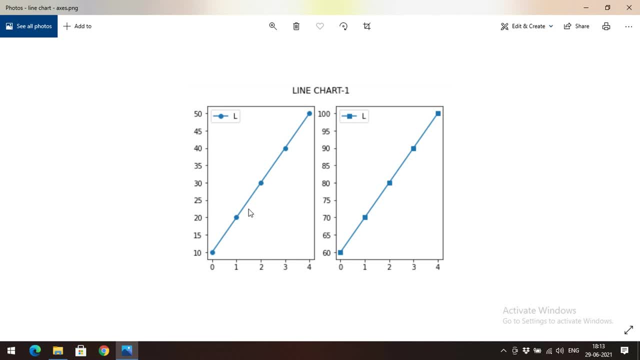 If you really understood my session, like my session, share my session with your friends and don't forget to subscribe to our channel. Thanks for watching. Thank you very much.